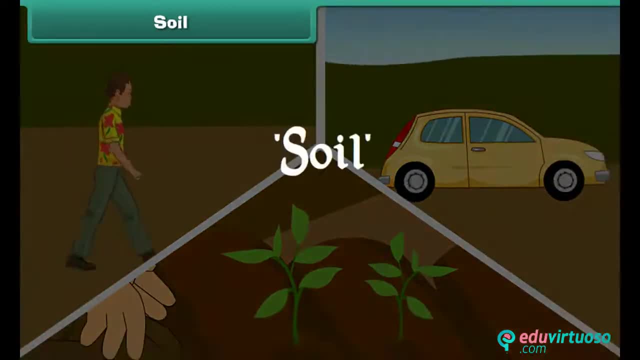 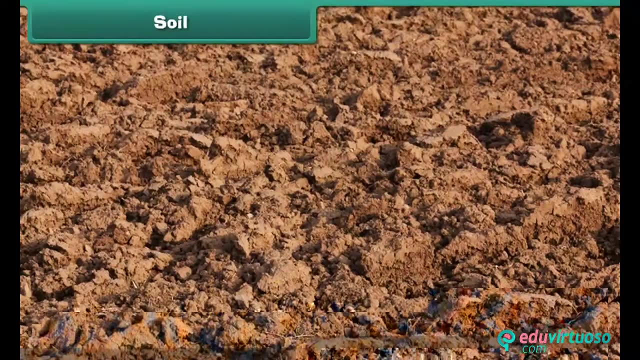 Wondering. what is it? It is soil. Soil is the uppermost layer of the earth's surface. It consists of a mixture of soil erosion and soil erosion. It consists of a mixture of soil erosion and soil erosion. It consists of a mixture of soil erosion and soil erosion. 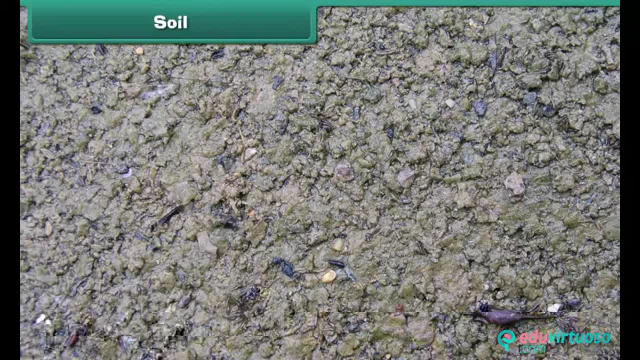 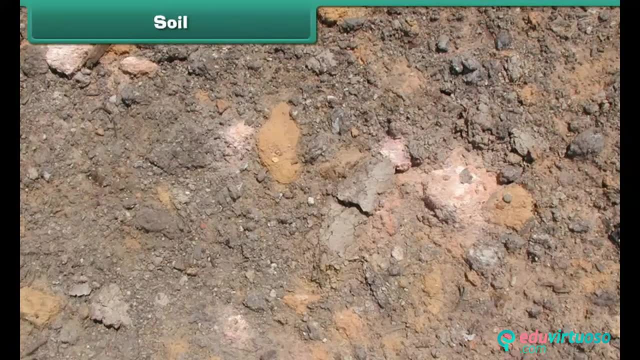 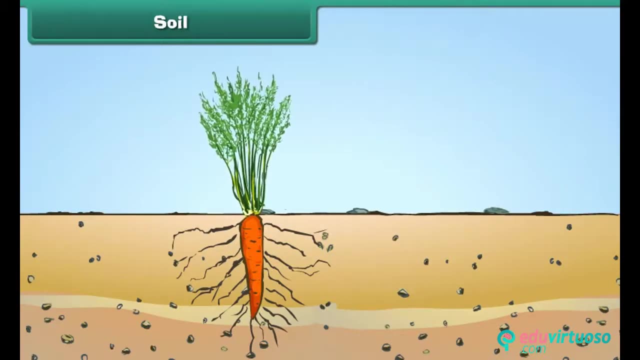 It consists of a mixture of rock finely ground into powder, water, air, minerals and a variety of living and dead life forms. It serves as a natural medium for growth of plants. Most soils contain four basic components: water, air, mineral particles and organic matter. 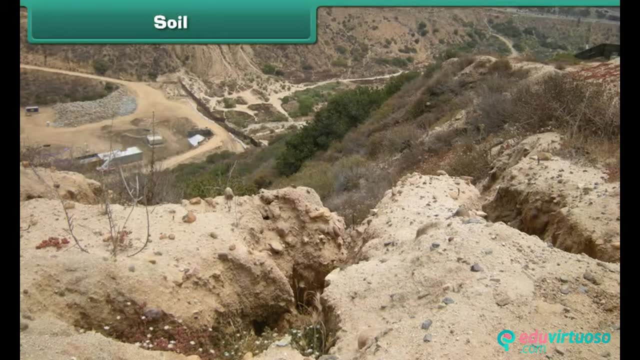 But the fertility of soil has decreased significantly. This is mainly because of the fact that soil erosion is a natural process. This is mainly because of the fact that soil erosion is a natural process. This is mainly because of the fact that soil erosion is a natural process. 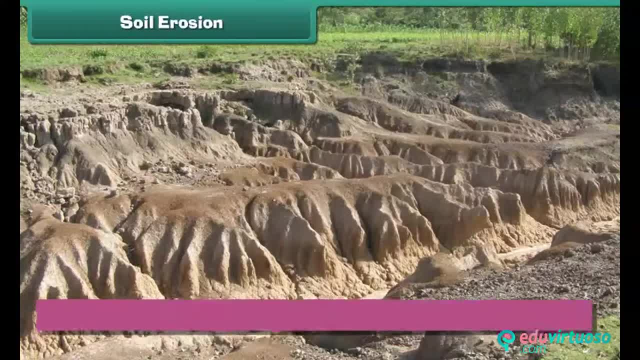 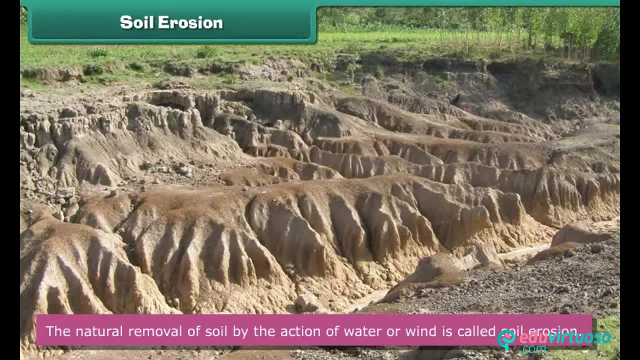 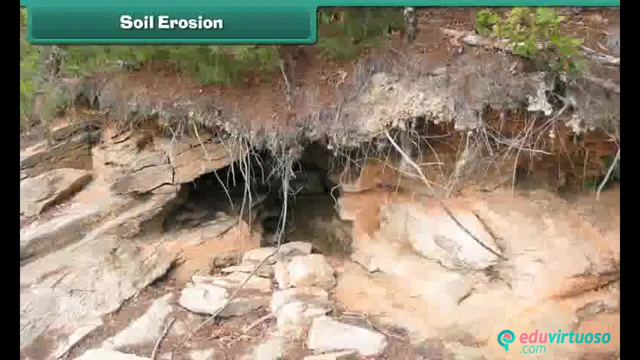 Come, let us learn about it. The natural removal of soil by the action of water or wind is called soil erosion. Look at the images: The disappearances of topmost surface and large ditches in the ground are the signs of soil erosion. 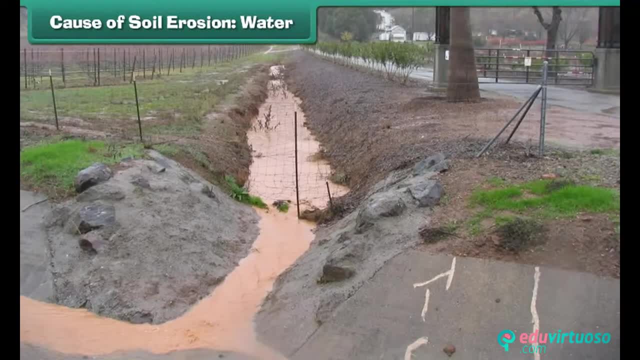 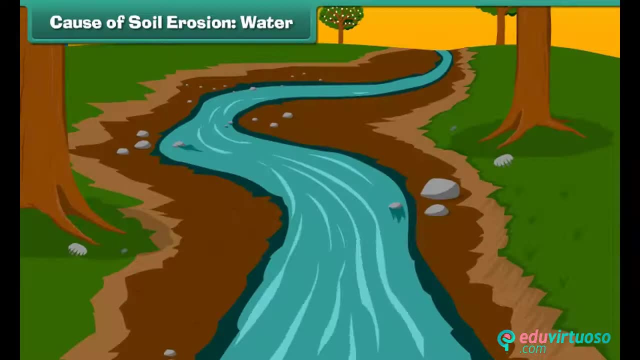 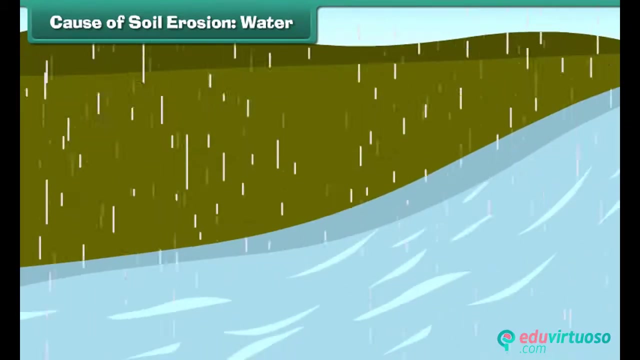 Friends, come let us know the factors which causes soil erosion. The most common factors are: The most common factors are: The most common factors are water and wind movements. water flowing through ground carries away soil with it. during rain, the soil particles are detached by raindrops. these soil 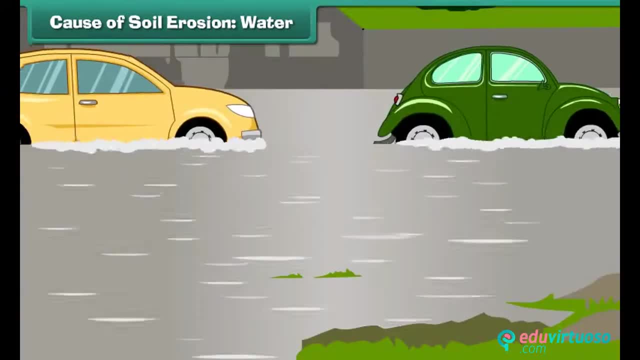 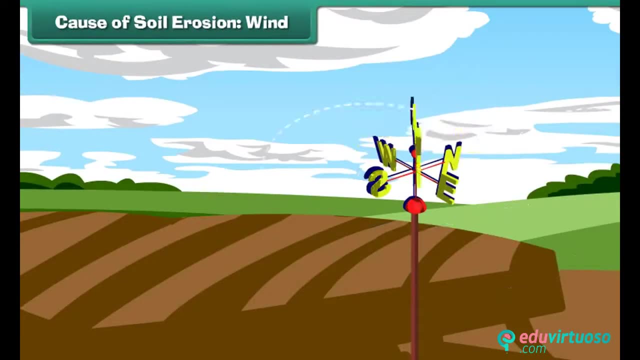 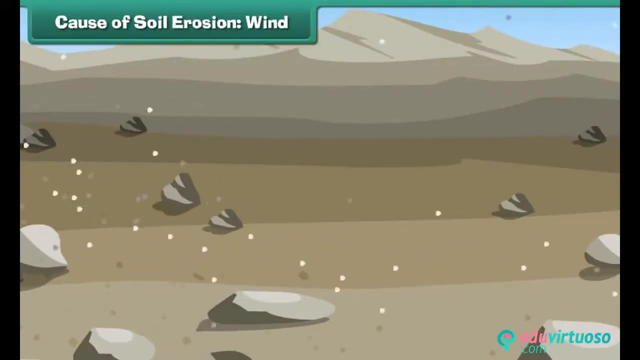 particles are carried away by the running water. floods are also the main cause behind the soil erosion. the other agent responsible for soil erosion is the wind. wind picks up the finer soil particles and takes it to the other location. during storms, the heavy wind takes away the bigger soil particles to 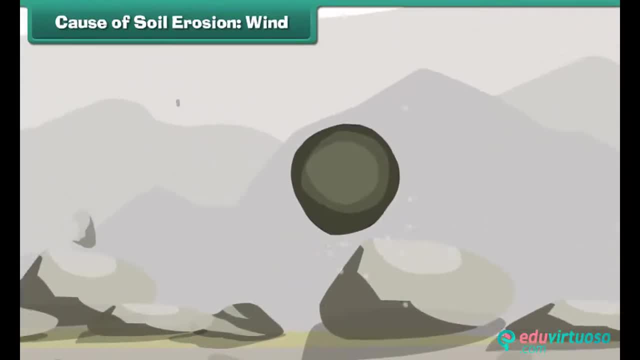 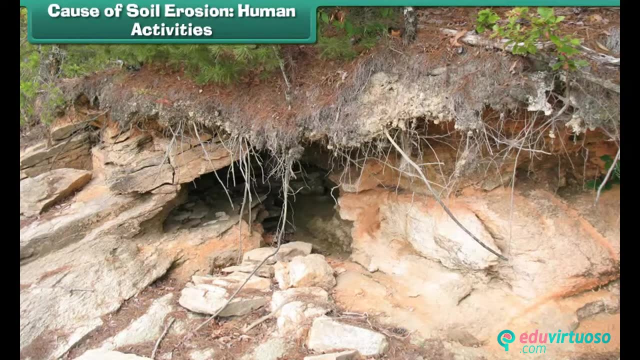 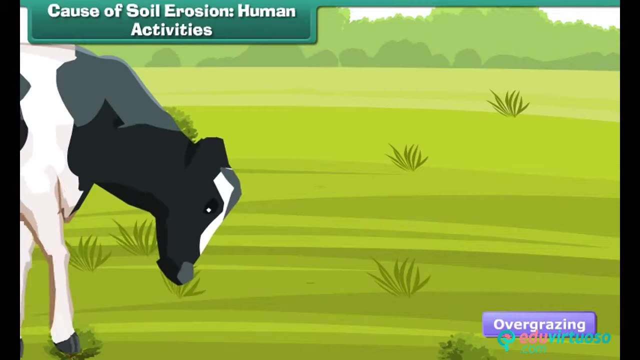 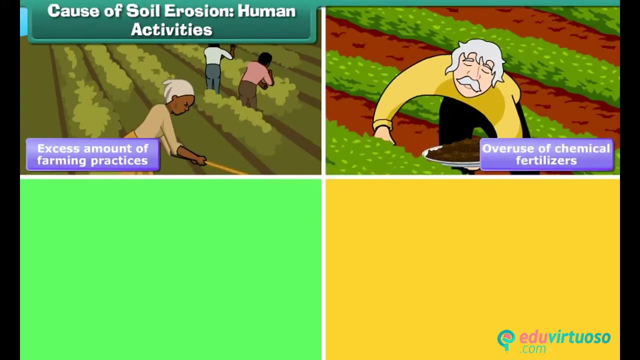 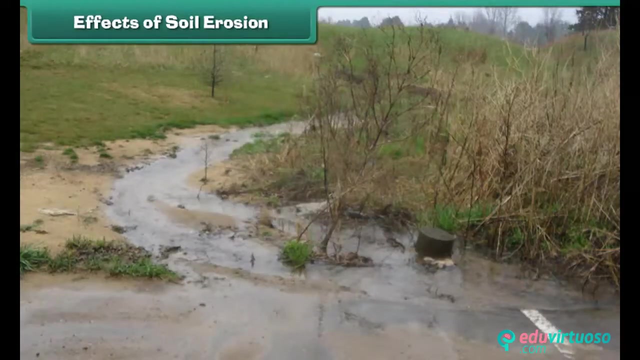 a distant place, and that causes soil erosion, though. soil erosion is in itself a naturally occurring process, but in many cases increased by human activities. some of these include deforestation, over grazing by animals, improper or excess amount of farming practices, trail building, overuse of chemical pesticides, fertilizers, housing, construction, mining, etc. soil erosion leads to many unfavorable conditions. 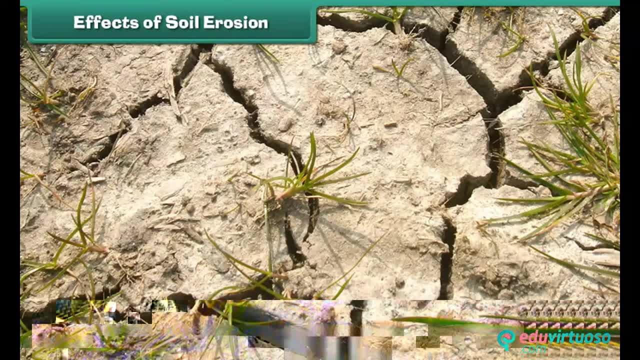 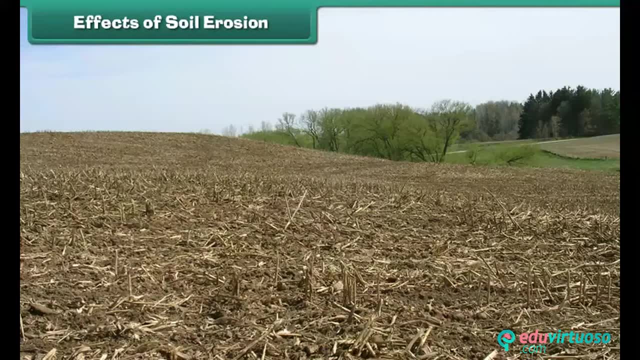 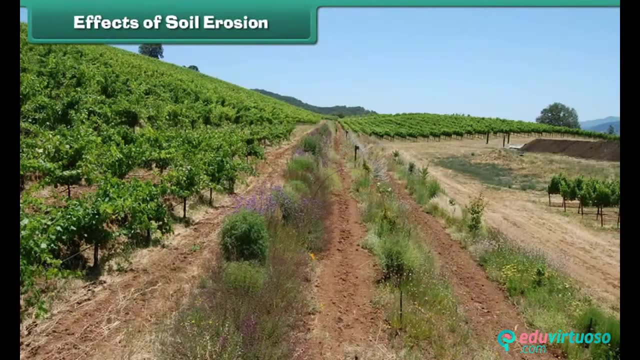 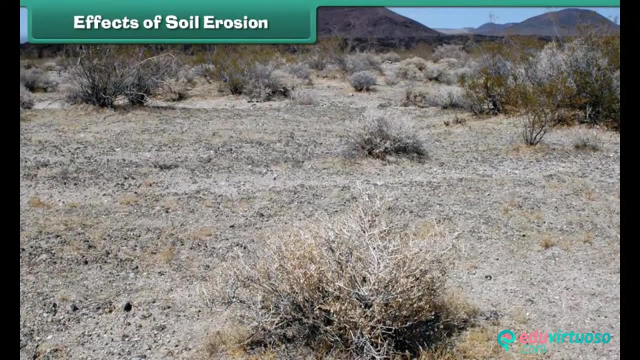 it results in the loss of soil and breakdown of the soil structure. it decreases the soil fertility due to decrease in the amount of organic matter. it also reduces the moisture content of soil, resulting in drought condition. decrease in soil fertility leads to decrease in the quality and quantity of the crops. thus, soil erosion affects the natural vegetation. 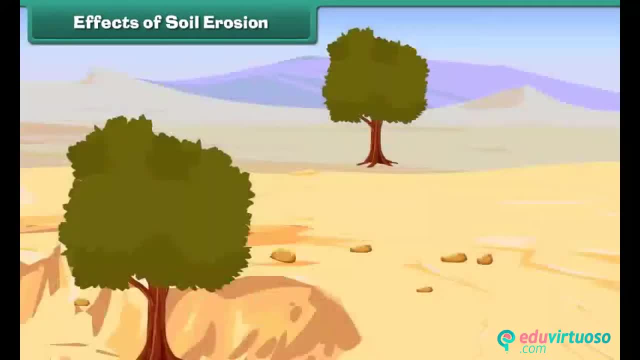 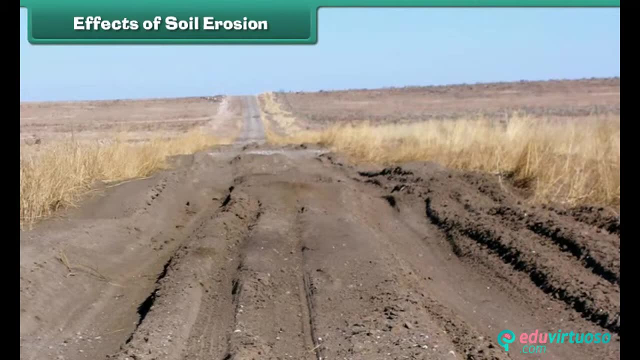 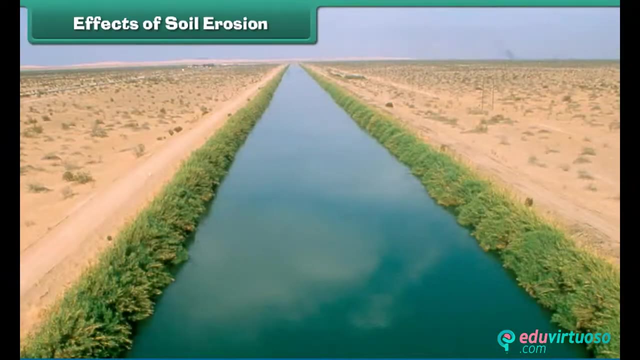 badly, which leads to transfer of fertile land into a desert. due to soil erosion, the soil shifts and accumulates on the roads and streets. this blocks the driving and results in accidents. it also blocks many irrigation canals. it increases the risk of flooding. the erosive reopenment of the monsoon seasonpeselsirts trying during fall for high be inastesin ocean. 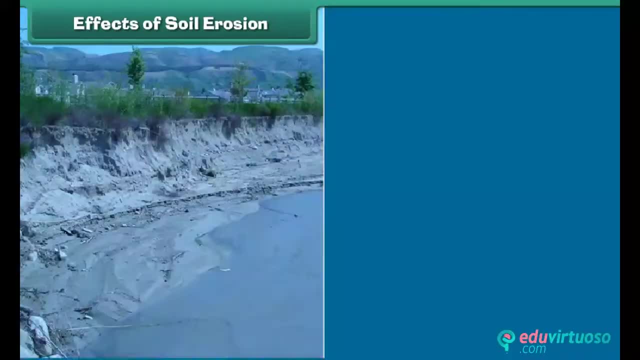 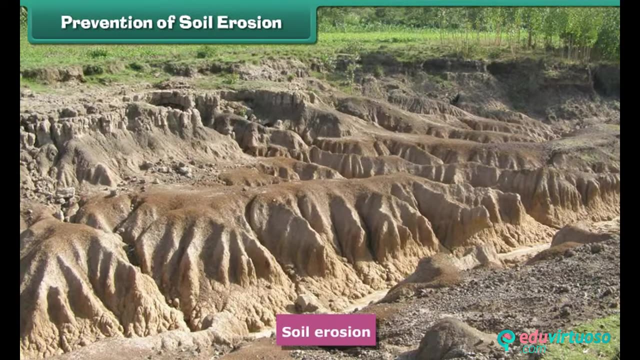 contamination photography. water collection rate, air raising, Bisadee under water control, Eroded soil deposits in water resources like river lake, etc. and pollute them. Soil erosion is a major environmental problem. It has affected all over the world, from forests to deserts. 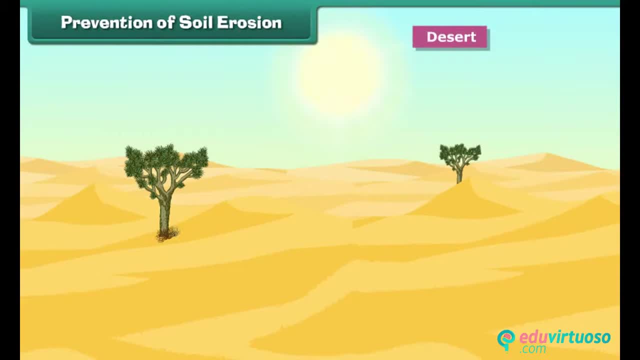 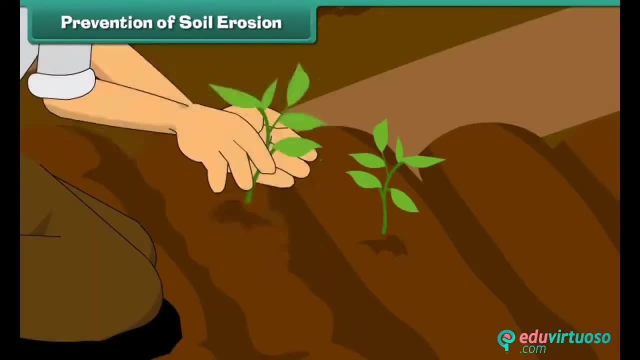 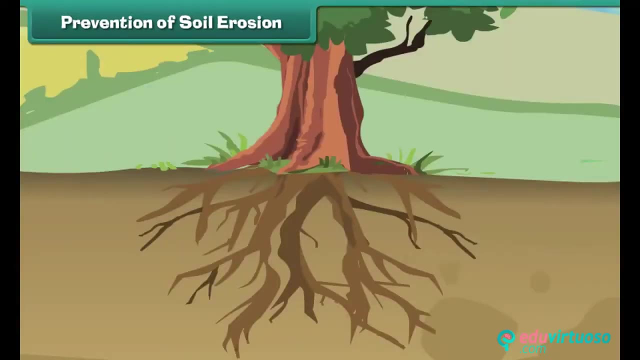 Thus it's the need of the hour to conserve the soil by preventing the soil erosion. There are many ways of preventing soil erosion. One of the most common ways is to grow more and more trees. The roots of trees hold the soil firmly and do not allow it to wash away easily. 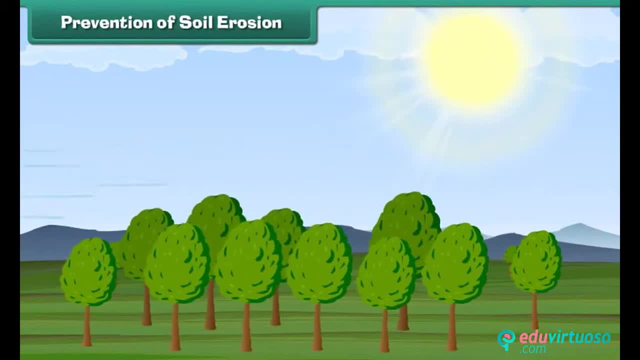 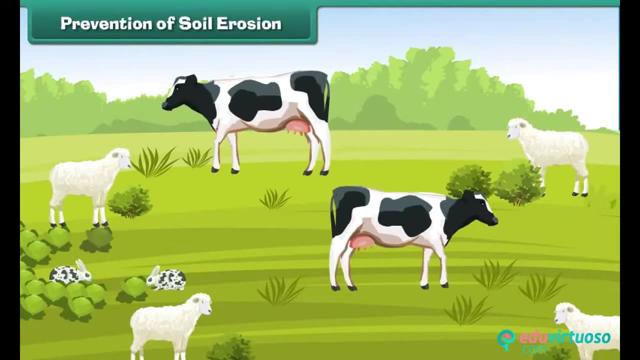 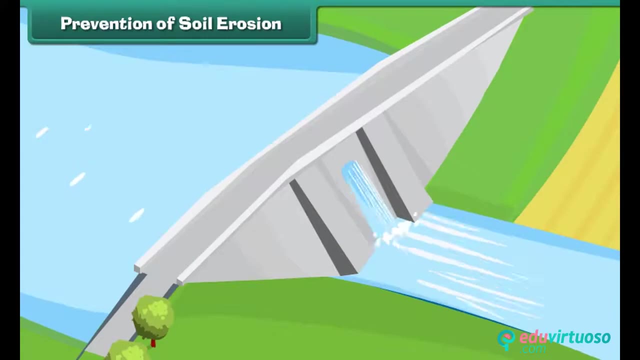 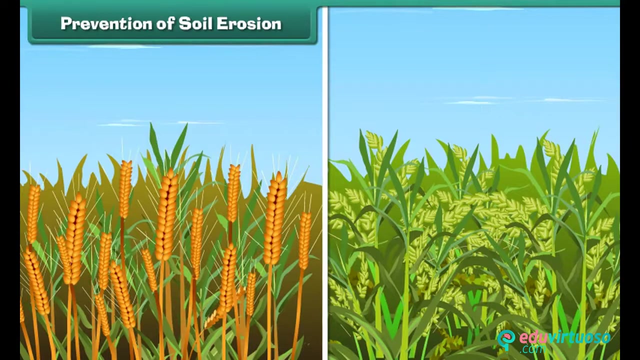 Trees planted across the wind direction protect soil against the high-velocity winds. Controlling overgrazing of the land by animals also controls the soil erosion. Building dams control soil loss. Some modern techniques of farming need to be practiced. For example, different types of crops should be grown at different times on the same land. 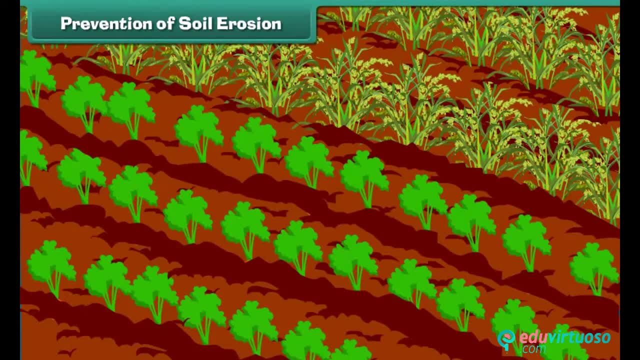 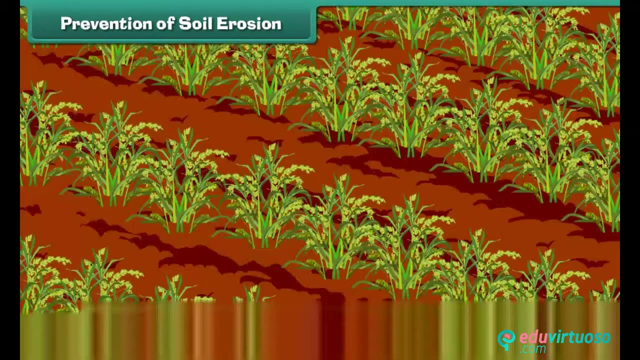 Different types of crops should be grown in the alternate rows in the same land. These practices control the loss of soil and increase the fertility of soil. Remember, friends, soil is a precious natural resource and it is our duty to conserve it for keeping the environment healthy.